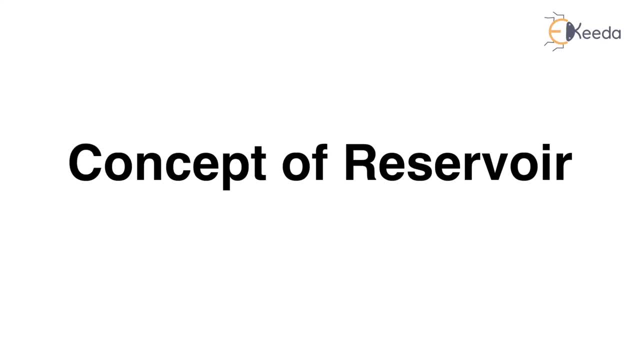 So, while designing the hydraulic structure, the first thing or the important thing is to design the hydraulic structure. The second element is the reservoir. So, before construction, constructing any type of a hydraulic structure, we need to construct or we need to investigate the reservoir properly. 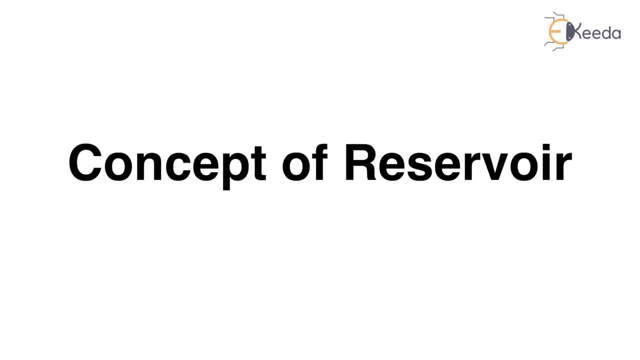 Reservoir is the open area or open watershed in which we are going to or, through the various sources, through the rainfall, the water is collected. Reservoir is going to be stored so that, after storing this water, we are going to construct the hydraulic structure according to the demand and then we are diverting this water to the various fields or for the various purposes. 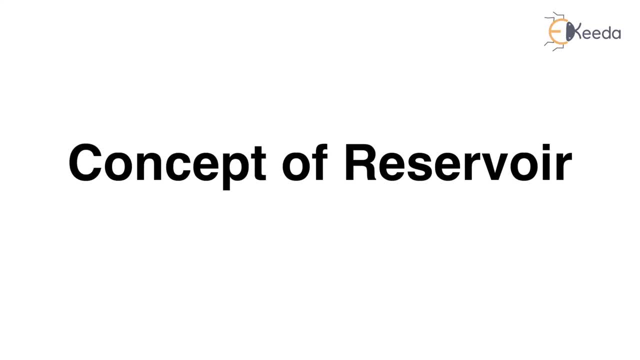 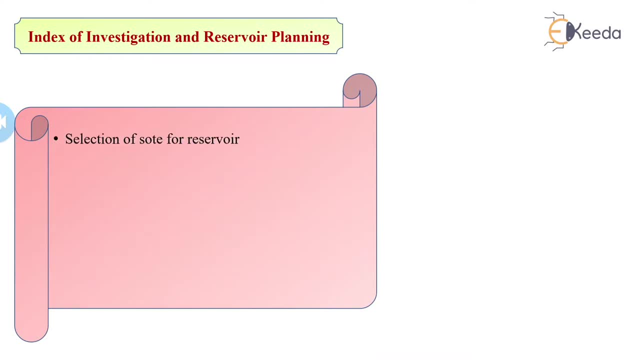 So let's see what are the contents which are included in this chapter: Index of investment, Restoration and reservoir planning chapters are selection of a site for reservoir, Then zones of storage reservoir, Then capacity elevation and area elevation curve of a reservoir site. reservoir sedimentation is there. 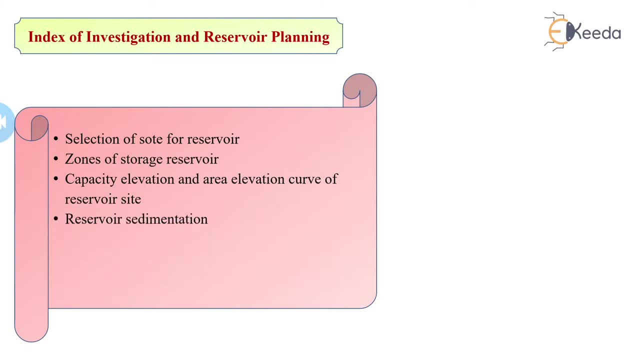 Then methods of controlling reservoir sedimentation. Then we have an evaporation loss. It's estimation of evaporation loss- And then the processing procedures. So all the procedures are included in this chapter. So here we are going to go through the phases. 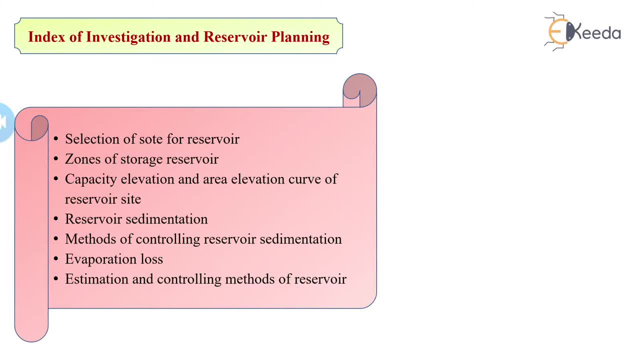 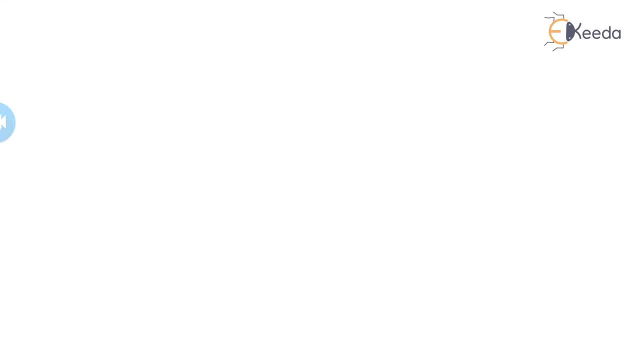 So the first one is the production oftag, a, called a clay or stone, Then the processing of type and type of the material and controlling methods of a reservoir. so what is the basic objective or main objective of this model or of this chapter? the first objective is to study. 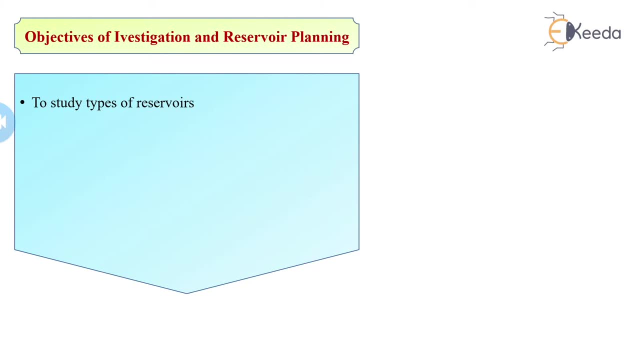 the types of reservoir. we need to know the. how many types of reservoirs are there? then, to study various site survey which is required for reservoir planning, to study about calculation of a life of a reservoir, to study storage capacity of a reservoir, to study concept of a reservoir sedimentation and to study the 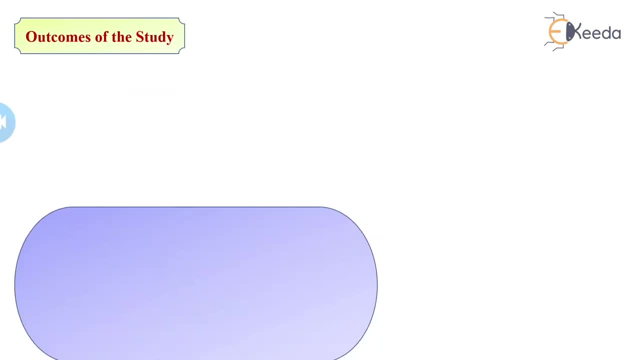 evaporation losses. after completion of this model, after completion of this chapter, the student will able to definitely able to classify the various types of reservoir according to the various use and according to the various need and concerns points. they will able to explain the zones of storage of reservoir. they will 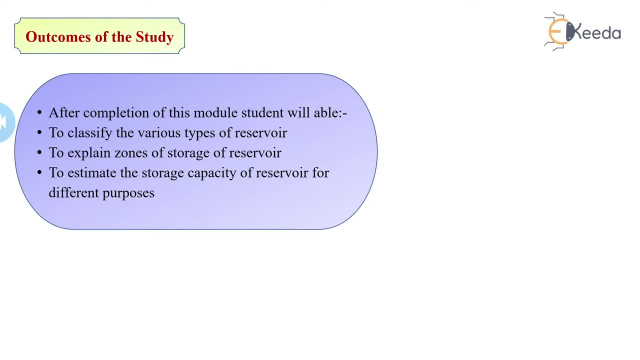 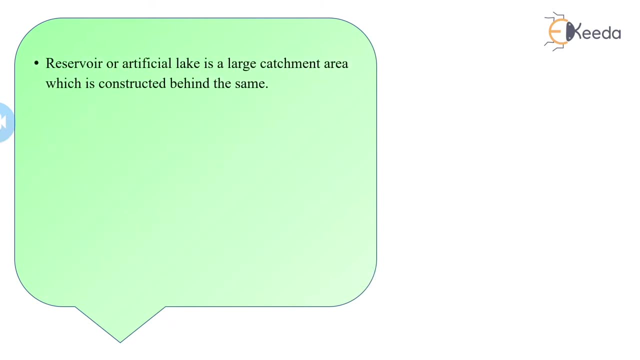 able to estimate the storage capacity of a reservoir for different purposes. so let's start with the introduction of a reservoir. see, reservoir is nothing but a artificial lake which is having a large catchment area, and it is constructed behind or behind the ane hydraulic structure, so behind any 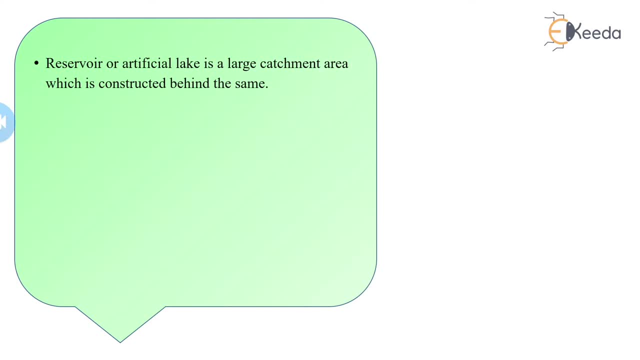 hydraulic structure means what? behind the time, behind the spillway, behind the gear, behind the, any obstructive area, any obstructed hydraulic area, so that we can store the water when there is a monsoon or there is a rainfall. so through the rainfall, the water will be collecting. 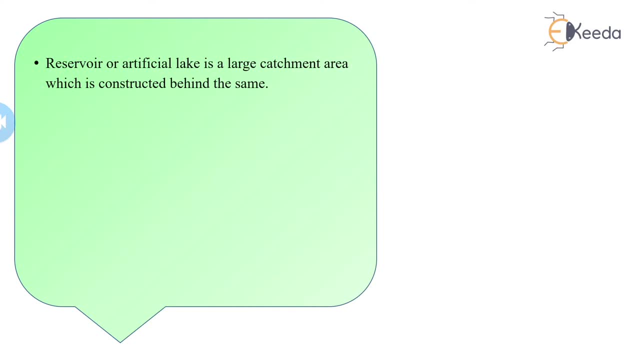 into the reservoir as well as through the various sources, through the mountains, through the small legs, through the streams. from this sources only the reservoir earth will get filled with the water. so classification of the reservoirs: see: basically, depending upon the purposes this reservoirs may be classified. so the first classification is the storage and conservation. 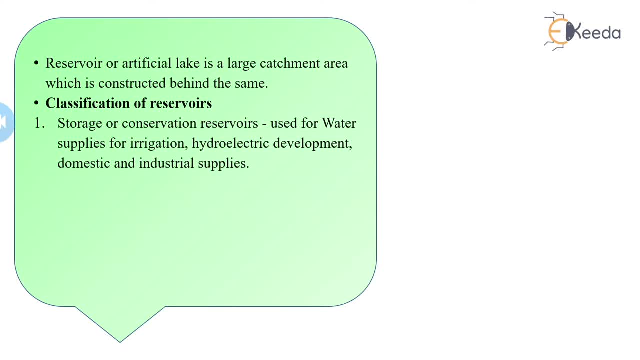 reservoir. so the name itself tell us that storage and conservation means this type of a Wesner voyer are primarily used for water supplies, for irrigation, then hydroelectric developments, domestic and industrial supplies. so in this reservoir we are going to store the water. the river does not carry the same quantity of water throughout the year, so it may carry. 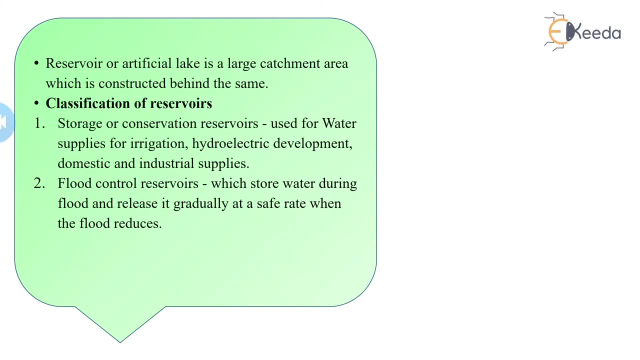 the large quantities in other part of the year. The storage reservoir is constructed to store the excess water during the period of a large supply- means during the rainfall only- and release it gradually as and when it is needed. So this type of a reservoir is used for storing the water during the excess period and after. 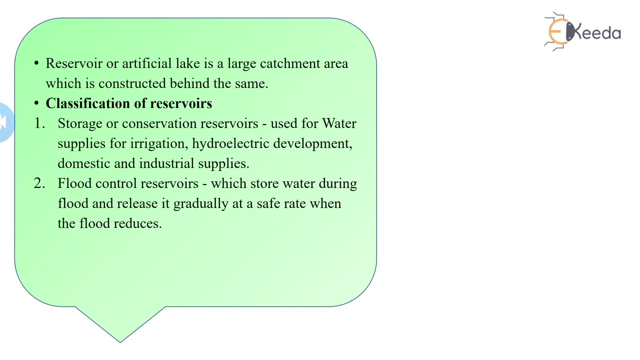 that gradually supplies this water to the various section, to the various field, according to their use. Then, second is the flood control reservoir. This is also called as a flood protection reservoir. These type of a reservoirs are those which store the excess water during the rainy season. 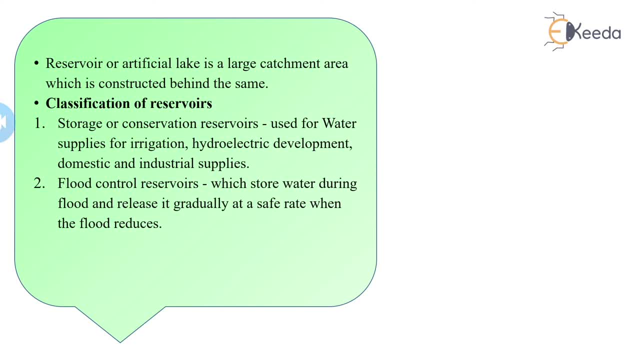 So this type of a reservoir is used for storing the excess water during the rainy season. Then, third, is that these installed and use a flood protection reservoir to store the water during the flood and release it gradually at a safe rate when the flood reduces, so that 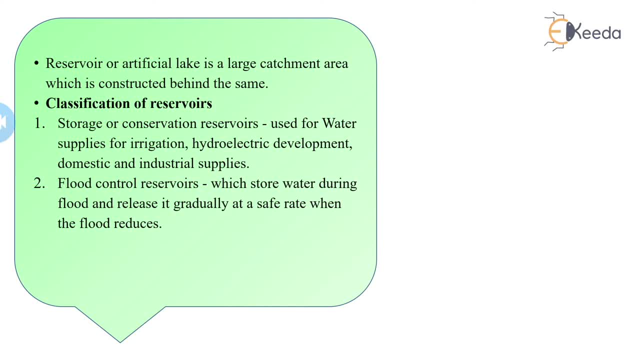 when this type of a reservoirs are constructed. So what happens during the flood situation? The excess amount of the water? if we don't obstruct and we don't distract that flow of a flooded water, then this flooded water will occupy the surrounding infrastructure of the reservoirs. Ledger said that it will dissolve in the floodwater till. this floodwater comes to the particulate in the mud storage reservoir, which will only support the mecabolic needs within the reservoirs. So it will last for many years, but then the flood water will be available in very wolf теam ministry per year or dinosaur empire. 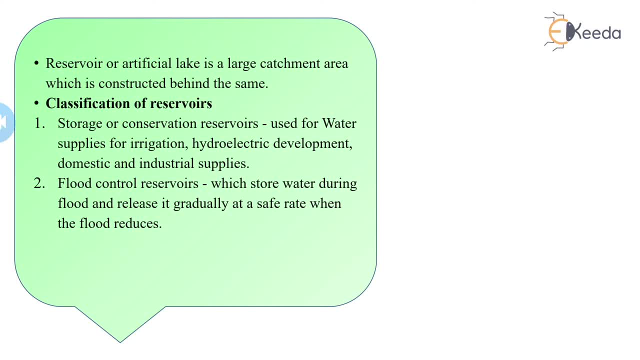 As such, this kind of a reservoir happens immediately, every two months, stored during the flood situation the excess amount of the water From Reno in all four years. when next year the flood water is transformed by the surrounding area near by the river side and the people who residing near by the 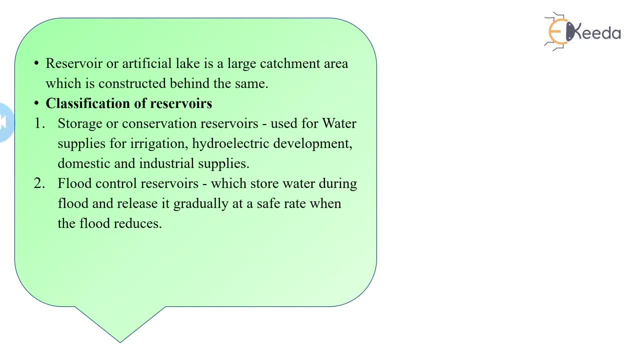 river side, they may get affected because of this flood. So for avoiding this situation, flood control reservoirs are constructed, So during the flood, the excess amount of the water is stored in this type of a reservoir and then it is safely discharged when the flood will be reduced. 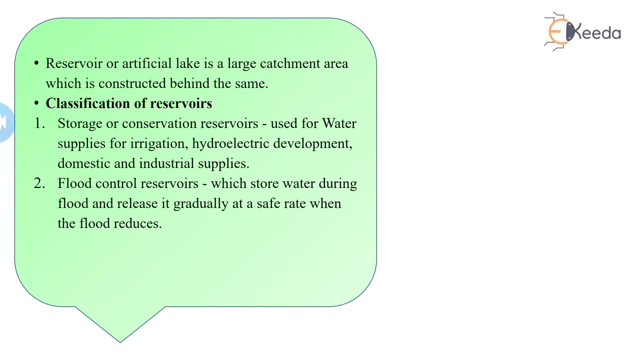 By the provision of artificial storage during the flood, flood damage downstream is reduced, obviously. So there are two pillars in flood prevention planning. First one is the riverbed stabilizing system, This planning for stabilizing the river channel from the upper stream down to the ancillary. 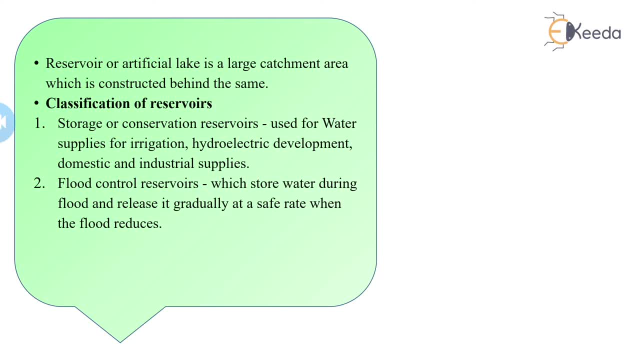 and flood deposition planning for causing the flood water to flow down without doing any damage. So flood control by means of a dam is part of a flood deposition planning covering the whole river system, and sometimes it shares part of a riverbed stabilizing system. So this is the flood control system. 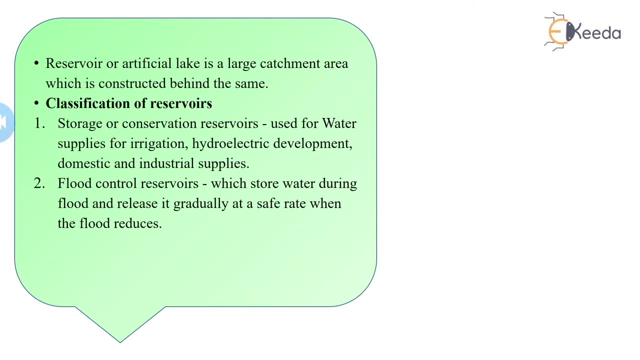 So this type of a reservoir plays an important role during the flood situation, if in future flood will occur. So this type of a reservoir helps, gives their best. Next is the distribution reservoir. This is the reservoir which is having a small storage area, or it is a small storage reservoir. 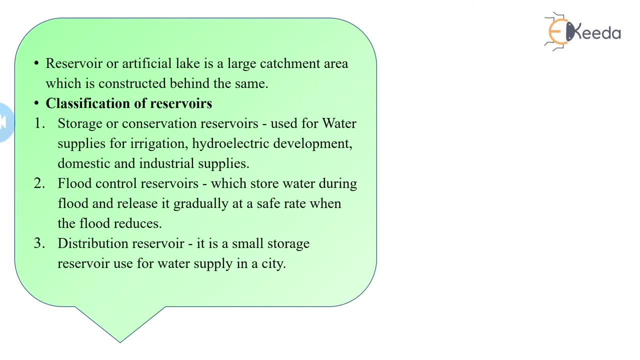 used for a water supply in a city. So the amount of the water that want to be supplied for the domestic, for the industrial purpose. So for this type of purpose the distribution reservoir is constructed. A distribution reservoir accounts for the varying rate of water during the day. 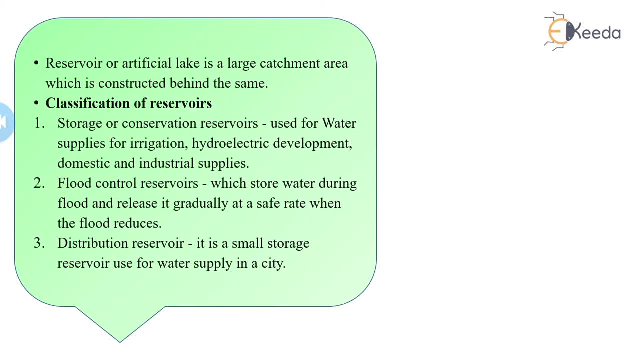 Such distribution reservoir permits the pumping plants and water supply. So this is the distribution reservoir. No matter what type of pamię is used, whether a water supply or not, the distribution solvent pumps the water done before actually entering a pond. make the mandea. 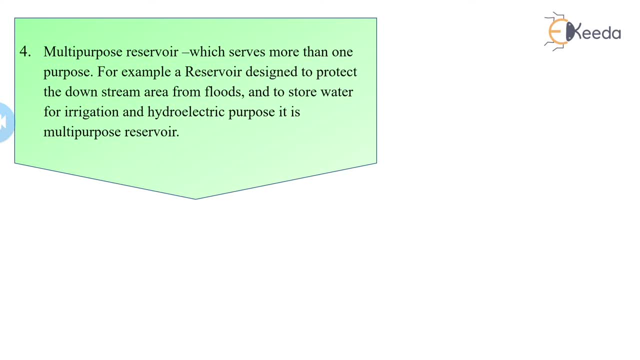 So it is made in continues with the distribution reservoir. Next, we have a multipurpose reservoir. So this multipurpose reservoir name itself suggest us that multipurpose means it serves more than one purpose. So, for example, the reservoir is used to sleeve Fachiamo Deixa, which is very popular. 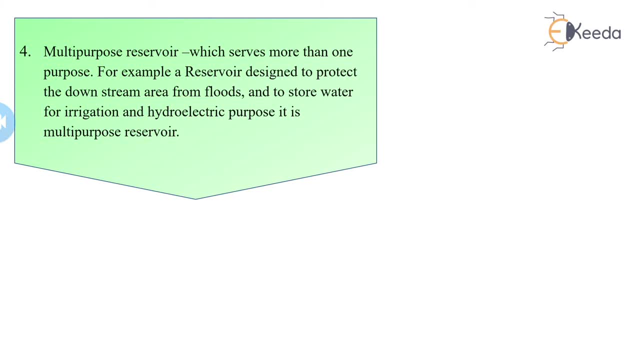 So we have saved all those units that need reduction in terms of eldery, totally without reservoir designed to protect the downstream area from the flood as well, as they are constructed to store the irrigation, to store the water which is required for the irrigation, for the hydroelectricity.